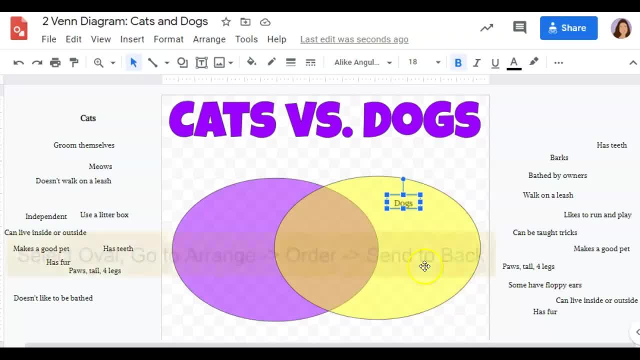 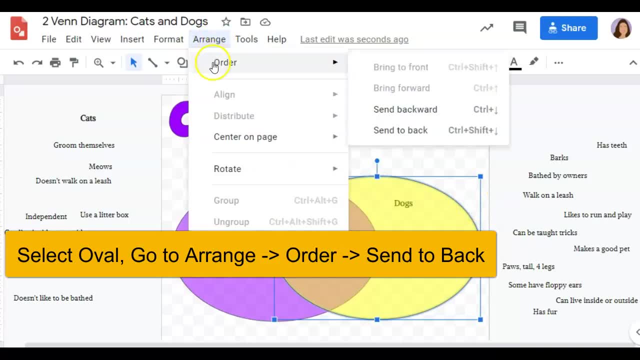 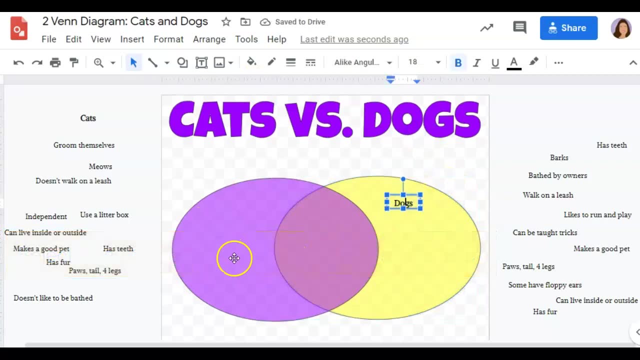 click on the actual oval so you see the border around it. selected Arrange order sentiment and click save. Now I'm going to go to my text box and I'm going to create my text box back now. you can see the dog is to black and you can move it. we can do that with this oval as well. 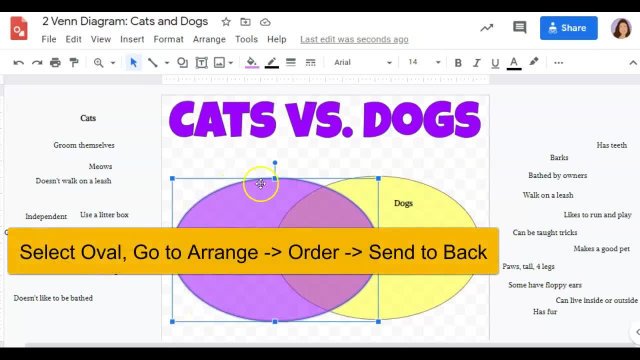 so again, click on the border of the oval so you make sure you're selecting the oval, because you've got the square around it. you're good, arrange, order, send to back, pause the video and please send both of your ovals to the back. now we're going to move the word cat over to the purple oval. 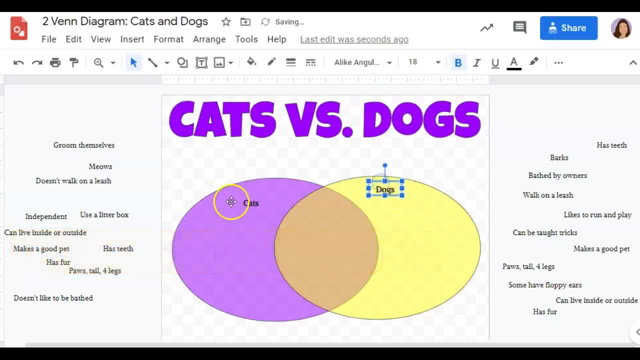 so we're doing- cats on one side, dogs on the other- kind of put it towards the top so it's visible and easy to see. i would even recommend maybe making it a bigger font or a different font so it sticks out again. just maybe a different font so it sticks out, all right. so next, anything they. 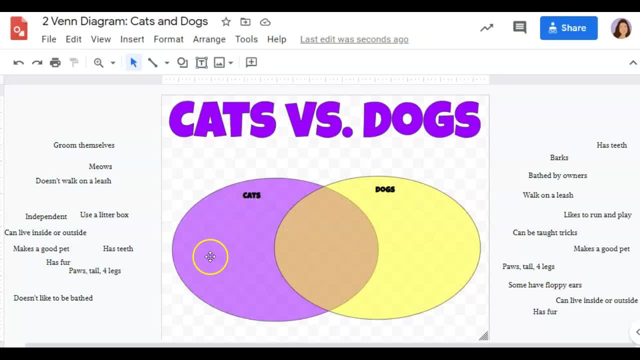 have in common with both sides goes in the middle. anything that's specific to cats, anything that's specific to dogs- all right, let's go with. has teeth, dogs have teeth. i'm gonna grab it and drag it. cats have teeth, oh, yes, they do. so instead of grabbing it there, we're gonna stick it in the middle. what do i do with this text box? 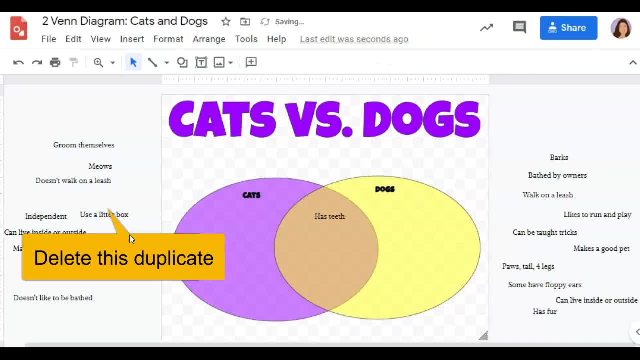 i click on the border and press the backspace or delete key. all right, cat's meow- that's a cat. the dog's bark- that's a bark, bathed by the owners. anything about bathing by owners? nope, they actually groom themselves. so we're going to grab and drag groom themselves. 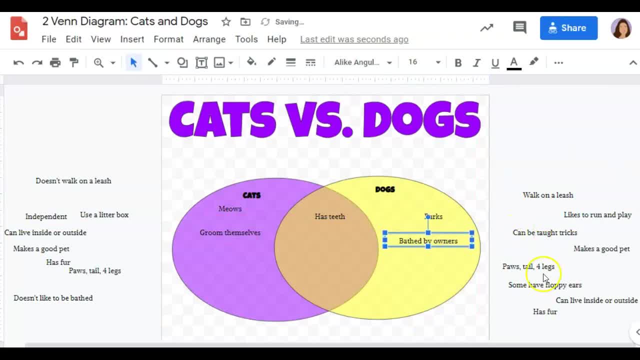 your job is to continue working with these shapes. so really quick one more time. dogs have fur, but wait, cats have fur also. so this time again because they both have it. it's sorry about that. undo wrong one, because they both have fur, where does it go in the middle? so if they both have it? 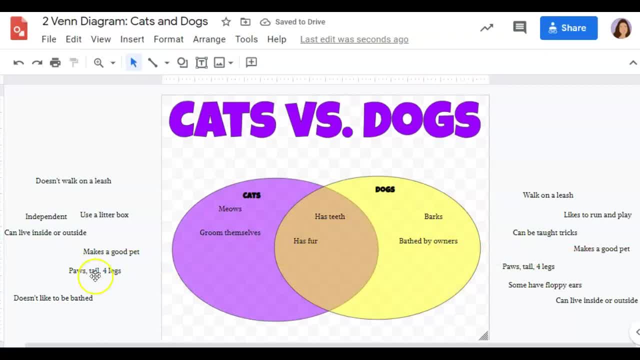 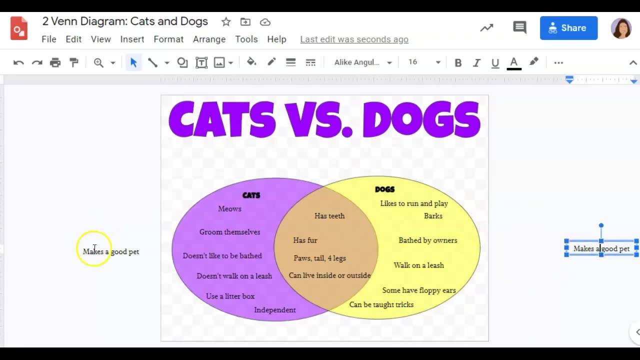 and delete this one, because they both have it. it's going in the middle one more time. they both have paws, tails and four legs. it's going in the middle because this one has paws, tail and four legs. your job is to finish the venn diagram. so one more time makes a good pet. makes a good pet.